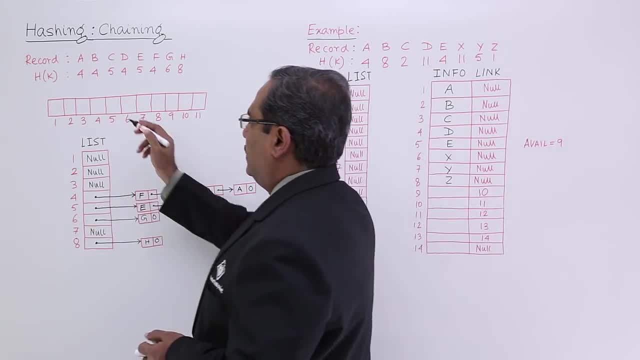 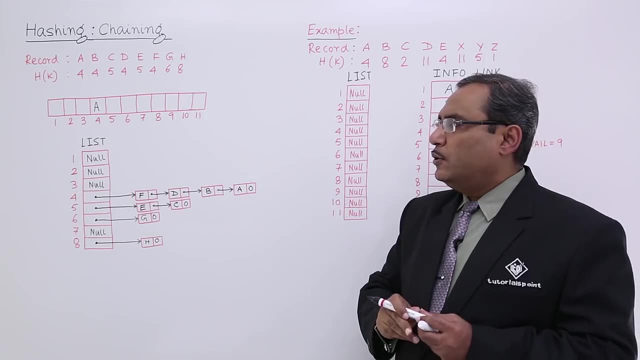 be stored at the location 4.. So H of K of A is 4.. So I am putting A here. Now B should be stored at the location 4, but the fourth location is preoccupied, So collision has. 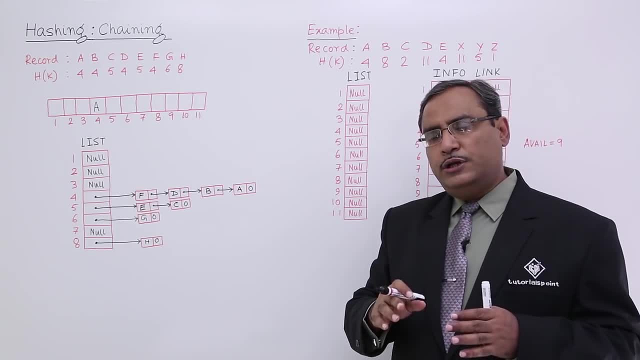 taken place. Here we are taking the linear probing as the collision. So we are taking the linear probing as the collision. So we are taking the linear probing as the collision resolution technique. So I shall go for 4, but it is occupied. 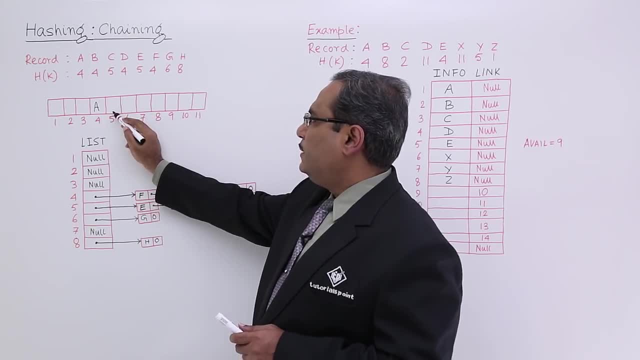 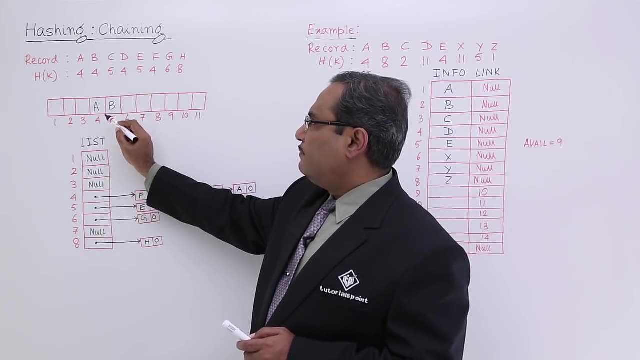 I shall. linearly, I shall search to the next free space. Let it be 5.. So I am putting B here, Then I am getting C. C is tending towards 5, but the fifth location of this array is preoccupied. So, due to the linear probing, I can reach to the next free space. 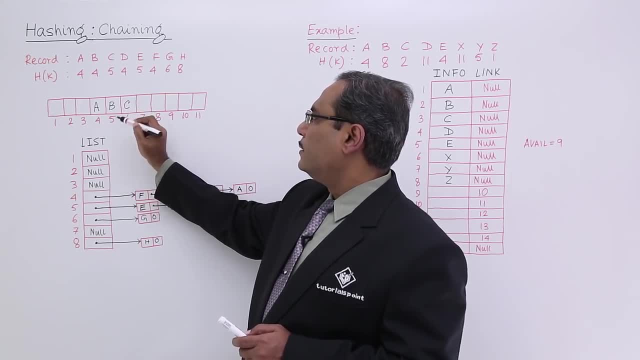 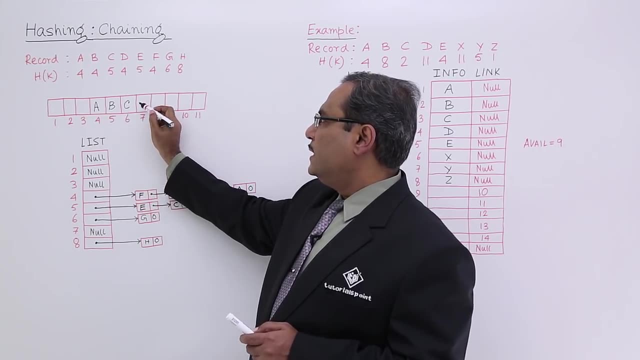 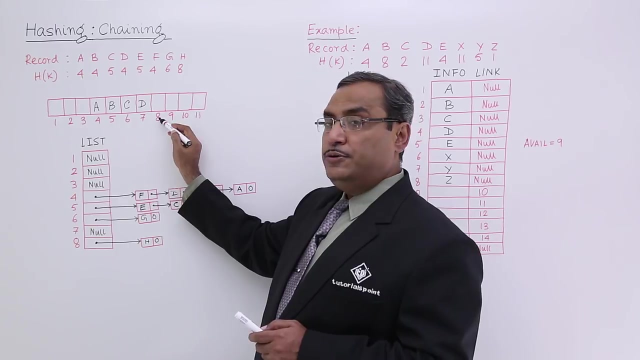 at a location number 6.. So C will be stored here, Then D will be pointing towards 4, occupied, occupied, occupied. So at the seventh place D can be stored, Then E at the fifth place: occupied, occupied, occupied. Due to the linear probing collision resolution. 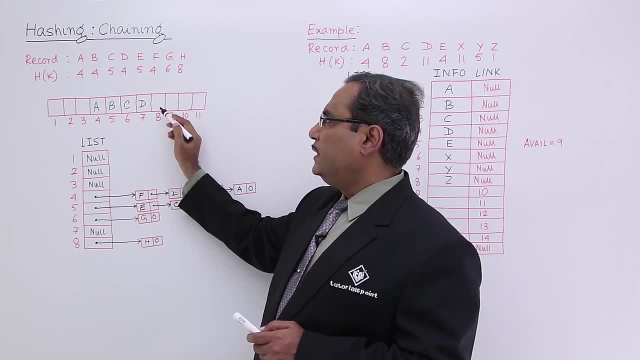 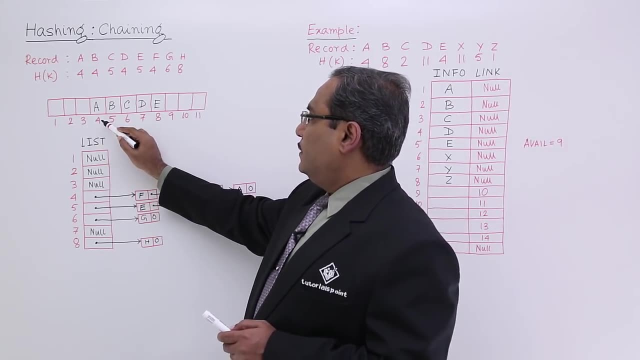 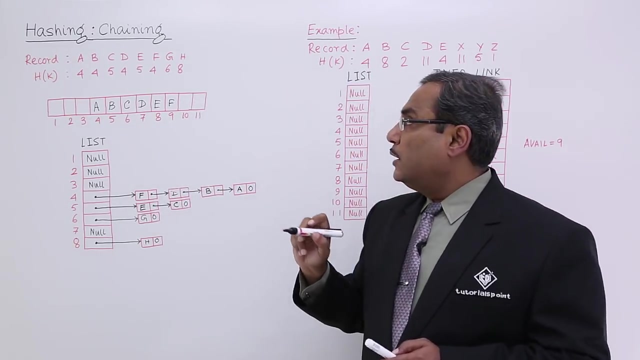 technique: linear probing. I am getting the eighth location free, So I am keeping E here, keeping the record E here. Now F 4, occupied, So I am keeping this one at the ninth location. Now we are going for the G, So G is pointing towards sixth location occupied, So G will. 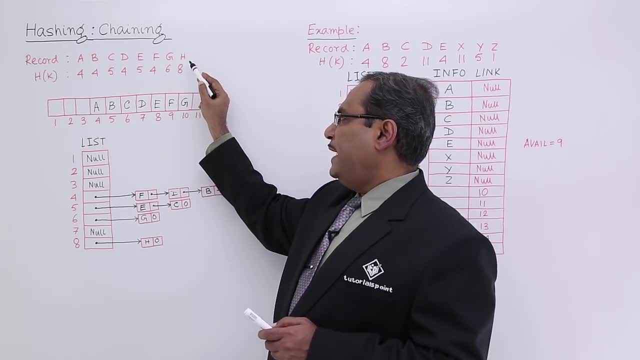 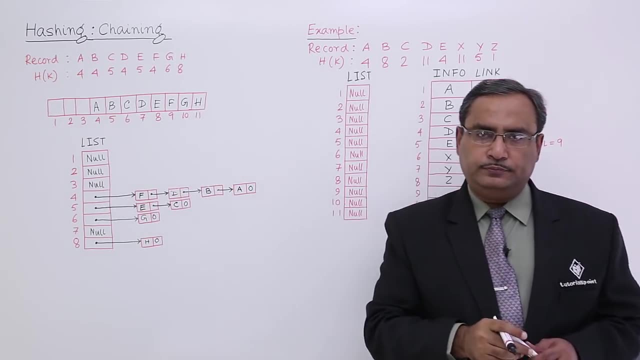 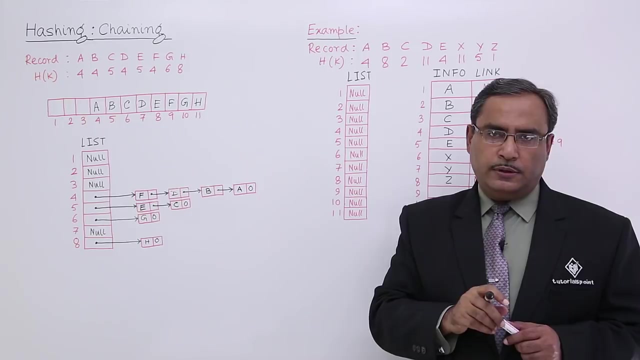 be stored here. Now I shall go for H, eighth location occupied, So H will be stored here. In this way, the values have got stored, So that is not an issue. Now let us search for G. Let us search for G. I am expecting successful searching here, So I shall go. 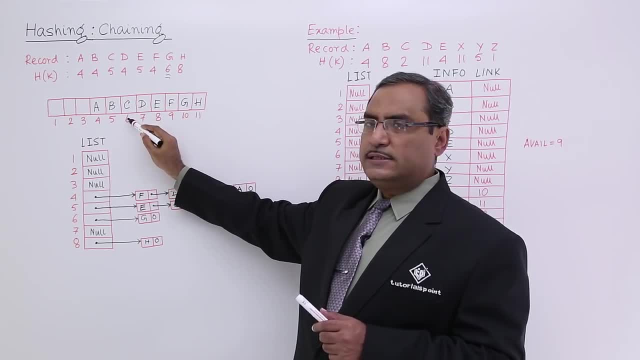 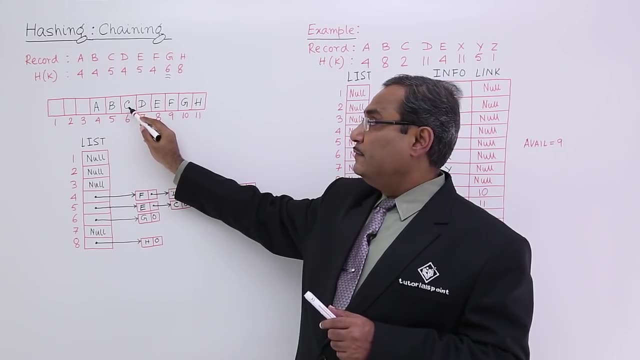 to sixth location, because this is a sixth, So I am going to search for G. I am expecting successful searching here, So I shall go to the sixth location. It is not G, But see C is having the H of K 5.. So it is. 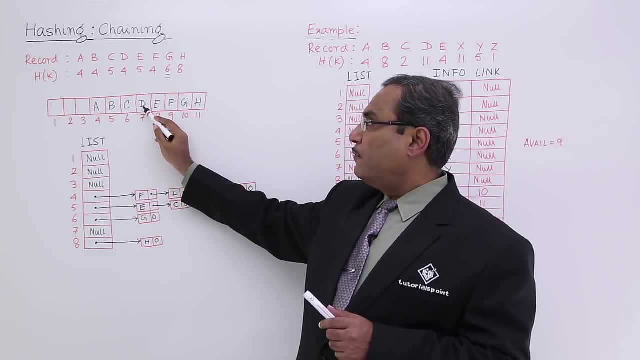 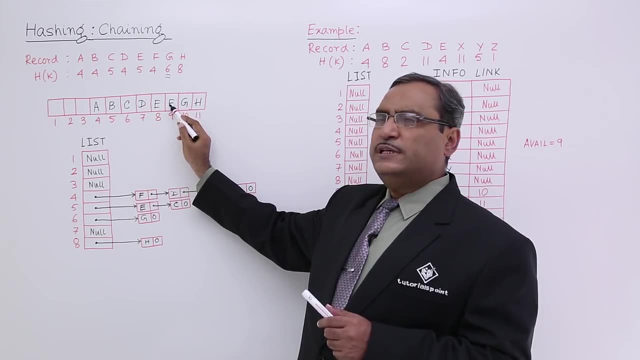 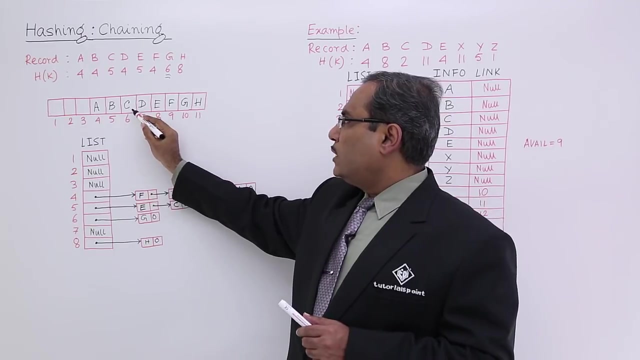 not G, But its H of K is 4.. It is not G, Its H of K is 5.. It is not G, But its H of K is 4.. But it is G. So successful searching has been obtained, But unfortunately, whatever. 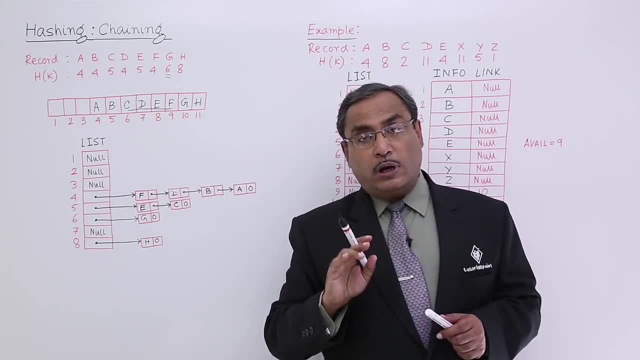 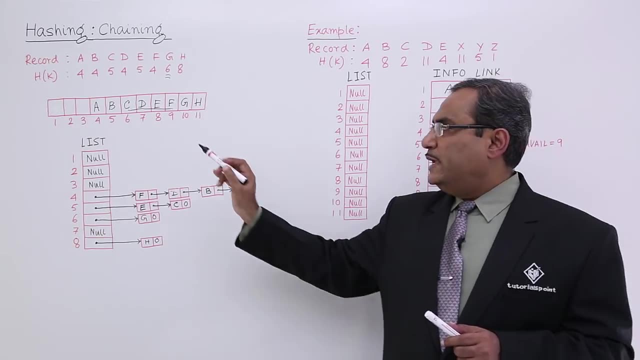 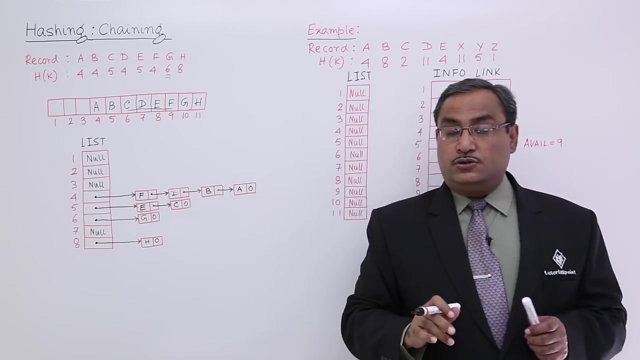 the nodes we have traversed, whatever the locations we have traversed and whatever the records we have traversed and matched, they are not having the H of K 6.. So here we are searching on those records whose H of K is not 6, either 4 or 5.. So, in case, 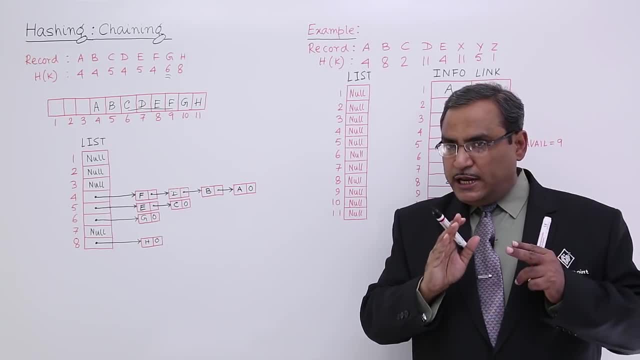 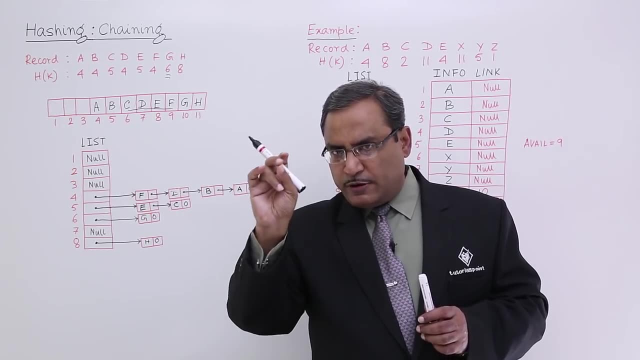 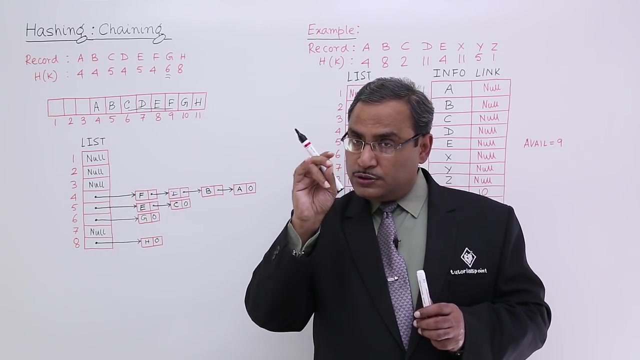 of. so. this is the problem here. But in case of chaining, whenever I shall search for a certain node, then I may have to traverse with different records their respective key values. But I can ensure myself that all those records having the key and the respective H of K will. 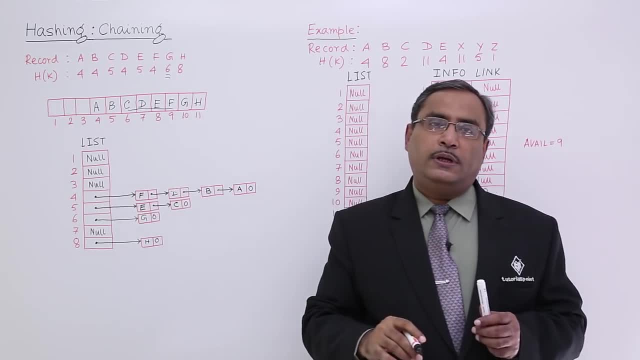 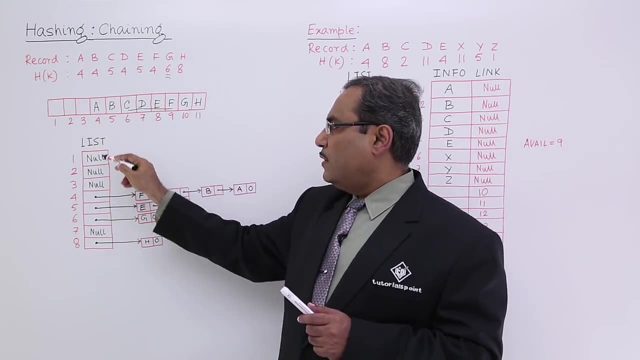 remain the same with the H of K of the search record. So that is known as the chaining. That means, if we apply this one, if we store these records in the form of chaining, it will be something like this: Look at here, So see, A will be at the fourth location. 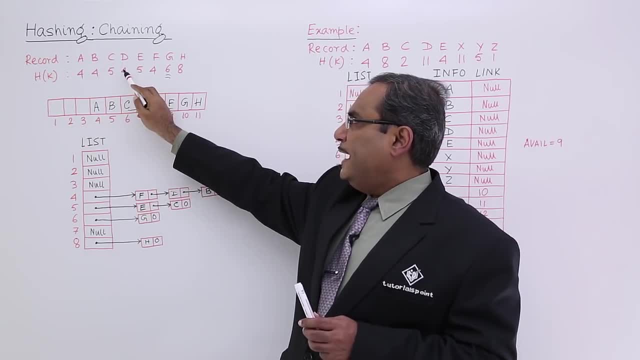 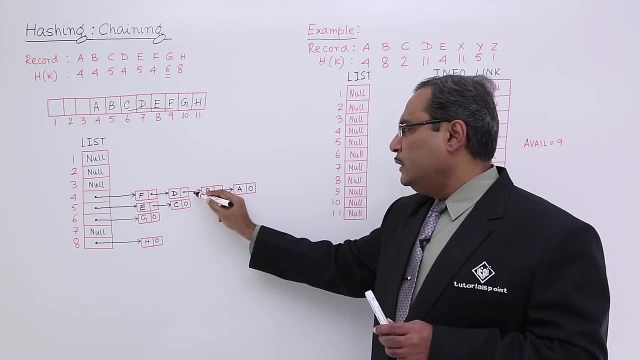 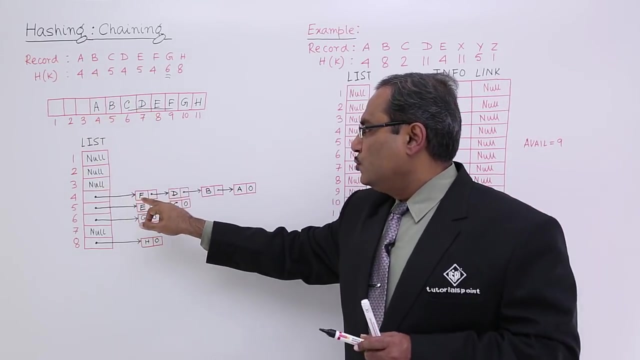 B will be at, the H of K will be the 4. D, H of K is equal to 4.. You see, we have kept for this 4, we have kept, we have kept all these records in a linked list format against 4.. So at first A will come, So A will be the first node. 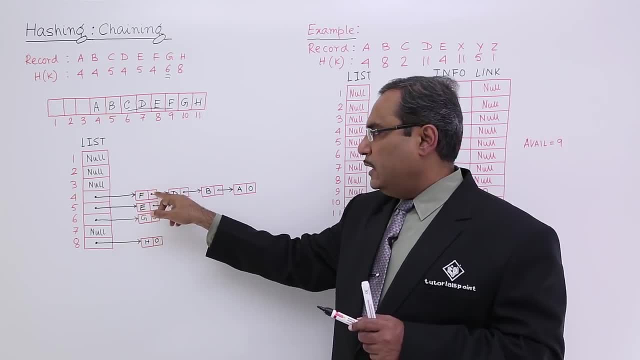 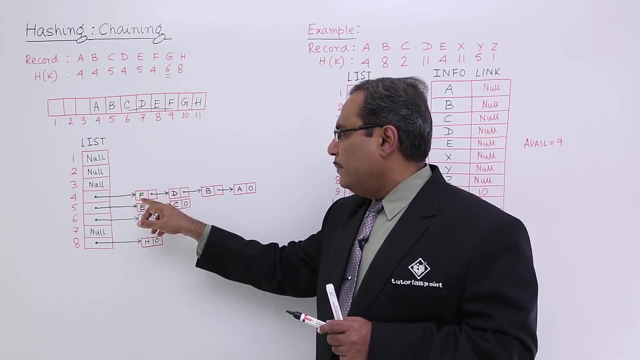 from the fourth location. So pointer will be there. It will be in the form of linked list, you know. So that means at the first fourth location I will be getting A, Then B will come, Then B will be prepended to A, you know, to insert. 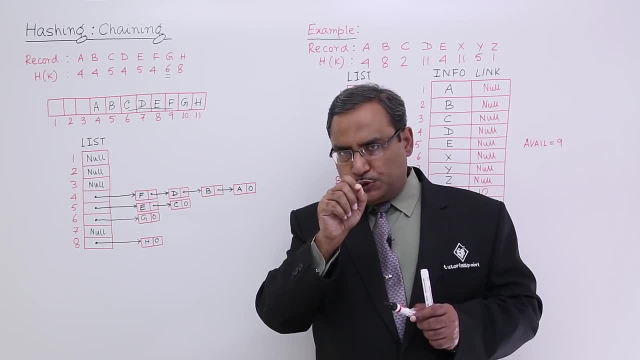 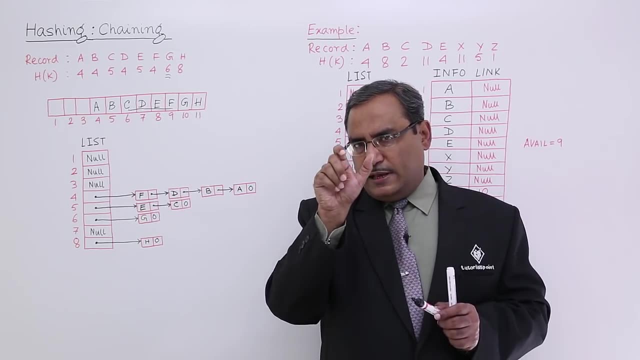 One node at the end of a linked list, That means you are supposed to traverse the entire list. But if you go for the prepend, if you go for the prepend, that means if you insert that node at the beginning of the linked list, you are having the constant time algorithm. 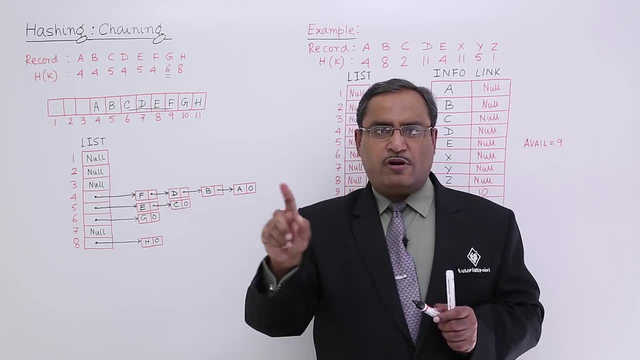 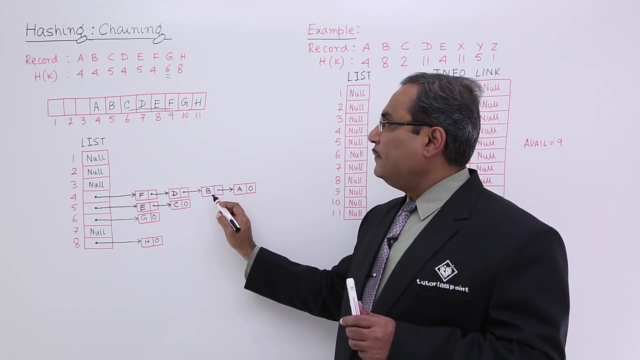 It need not to traverse the linked list, all nodes It need not to traverse, So that can easily be put at the head. So that is why at first A was there, Then B came, After B, D came, So it has got prepended. 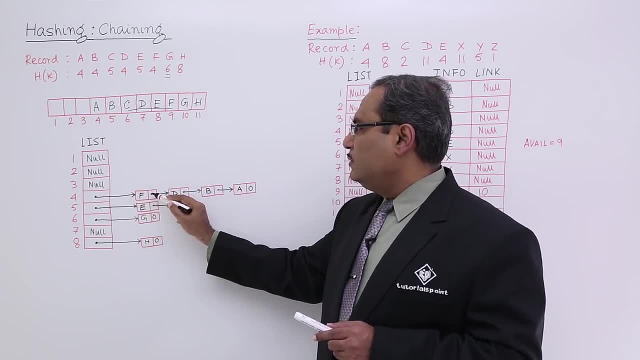 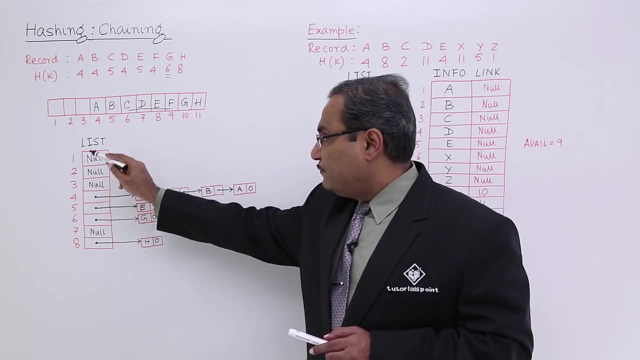 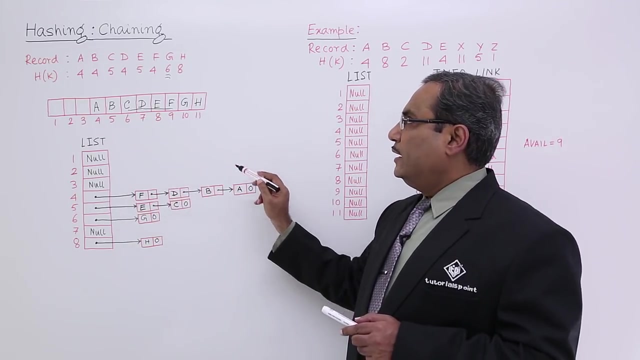 Then B came. So that is the ultimate chain And all these records are having. the H of K is equal to 4.. So from the fourth location of this list we are having the starting at this of this linked list And then I can traverse in this way. Now for E, for 5, I